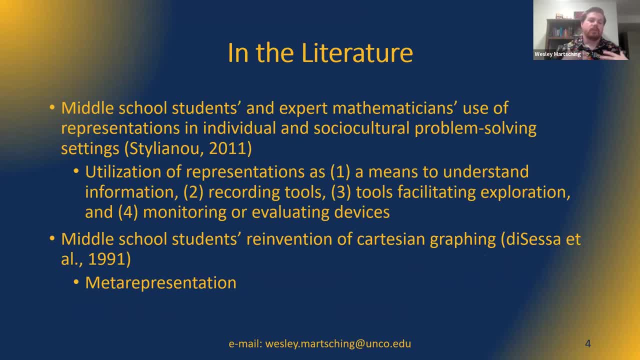 And two of the studies, particularly the information That influenced my current work was Stylianou's research, which looked at representations as tools and problem solving. Stylianou determined that expert mathematicians and middle school students used representations as a means to understand information, as recording tools, as tools facilitating exploration and as monitoring or evaluating devices. The other study that really influenced my work was de Cesse's study from 1991, which looked at students' 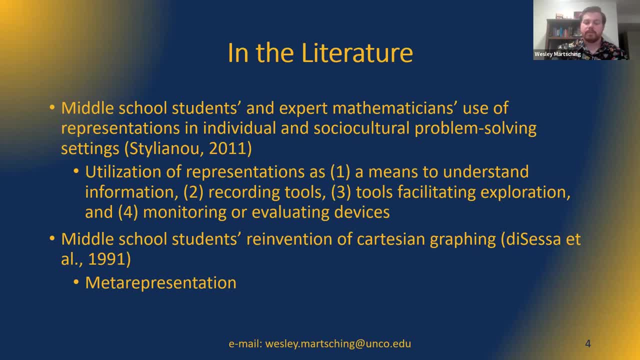 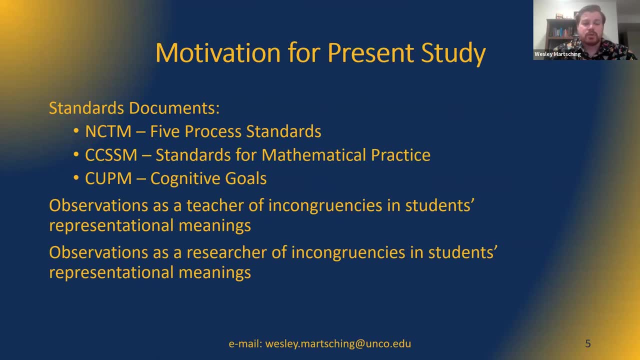 re-invention of the graphing representation Motivation for the present study. Representation is heavily emphasized throughout the standards documents And for me right now, the CUPM guide is really the main one that influenced my work, And also my observations as a teacher and researcher influence this, So I've noticed that my students and my participants in the studies will often create 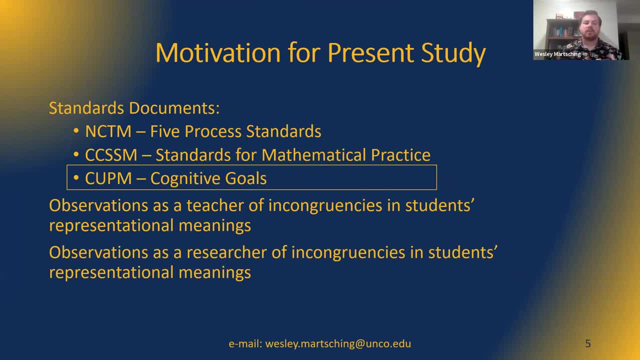 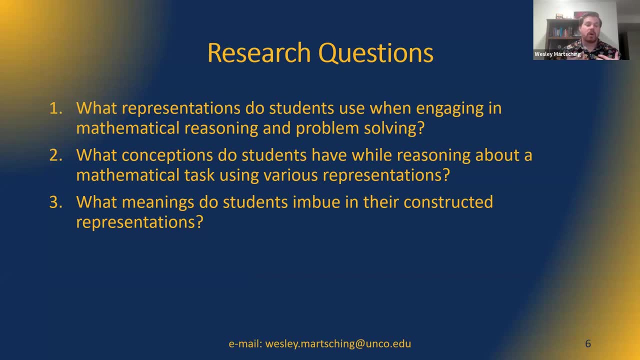 multiple representations for the same context, but the meaning for each representation might vary. So my research questions were: what representations do students use when engaging in mathematical reasoning and problem solving, What conceptions do they have when reasoning about a task using these different representations, And what meanings do these representations actually have for these students? 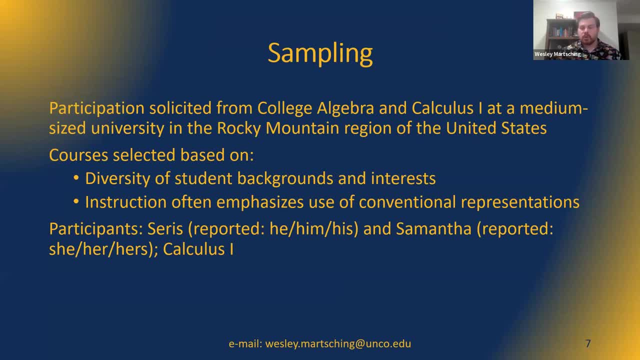 I sampled my population from College Algebra and Calculus I courses, because of the diversity of student backgrounds and their interests, and because instruction in these courses are really centered around more conventional representations a lot of the time. However, because this study occurred at the start of the COVID pandemic, I was only able to conduct interviews with two participants, Ceres and Samantha. 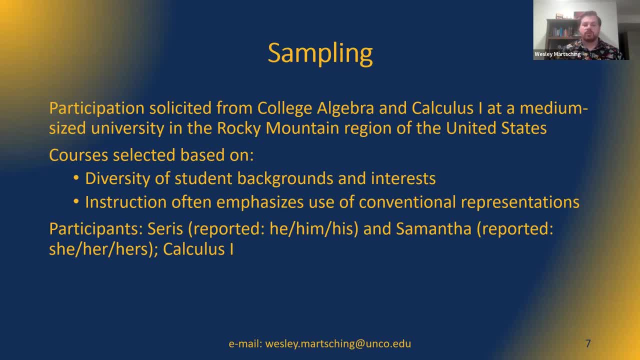 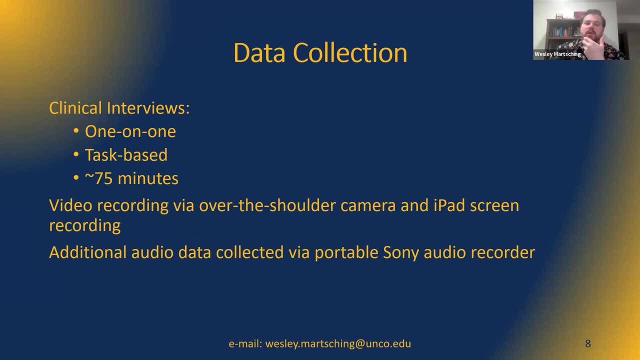 before we went fully online And both of these students were employed in Calculus 1 at the time of the study. Each participant- each student- participated in a one-on-one task-based clinical interview that lasted about 75 minutes. I collected data using over-the-shoulder camera and 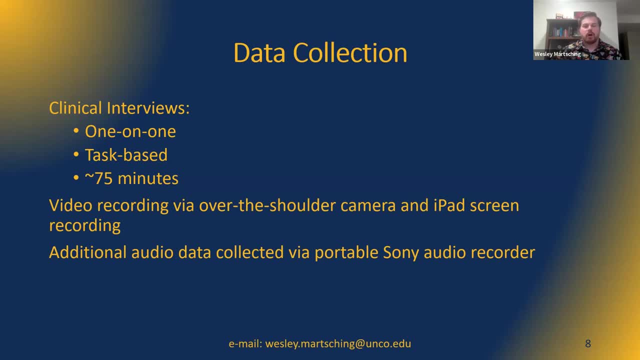 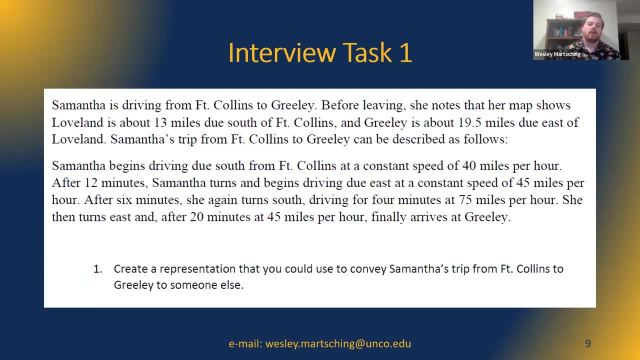 iPad screen recording and then I used an additional audio recording device just in case there were any issues with the audio from the camera. The study was comprised of two tasks. The first one was this task that depicted this car traveling from Fort Collins around Loveland to Greeley. I only realized, kind of when I was 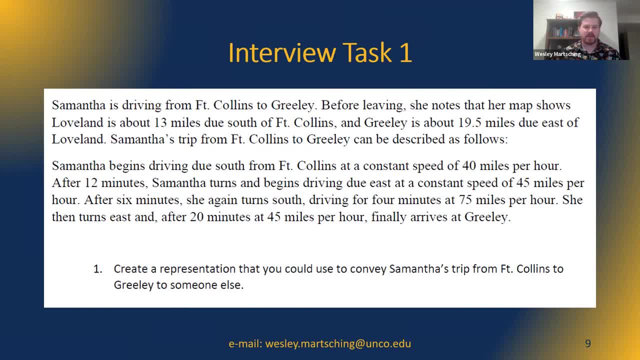 creating this presentation, that my participant decided to use the same pseudonym as the individual that I had put in this task. So when I refer to this task, I will refer to the car instead of the car. So I'm going to refer to the car instead of the car. 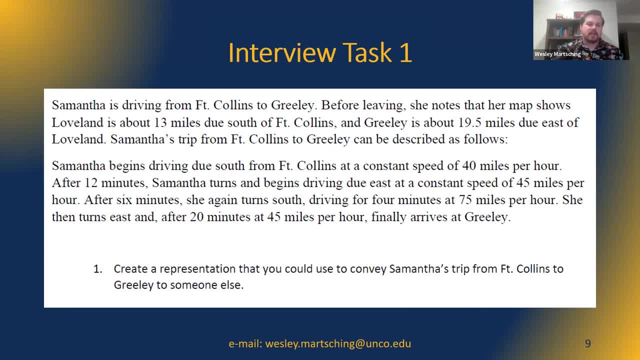 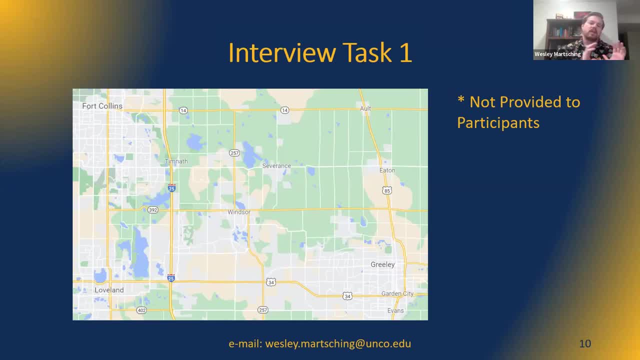 Samantha. But this was the first task and since both participants were from the Rocky Mountain region, they are kind of familiar with the orientation of these cities. They weren't given this map but it was kind of taken that they knew or were familiar with the area. 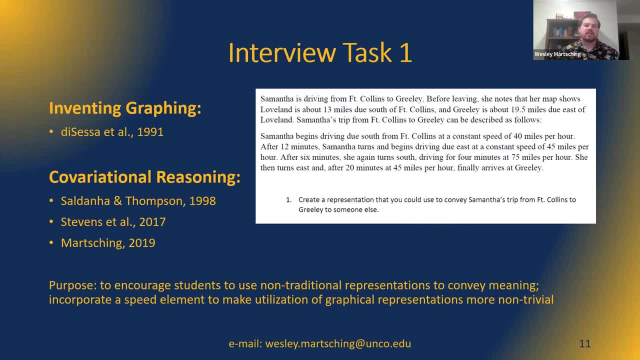 This task was modeled after several tasks that have been looked at in co-variational reason literature, because it really often challenges students' notions of what they're doing and how they're doing it and how they're doing it. So they looked at these three main tasks. dozens of graphical representations. 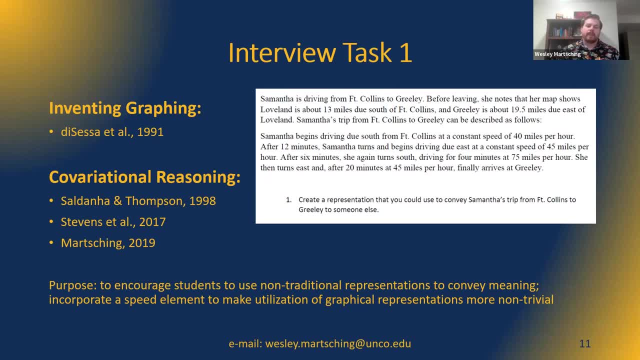 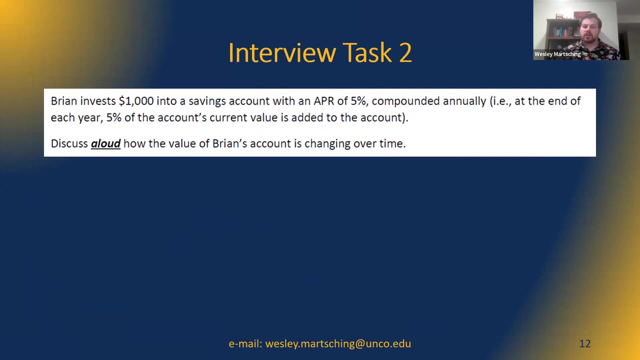 of these cities and they began looking at how they could dniCOORD nosebars Samantha Really quickly. in this part I'm going to show you the second task, which is one of the other tasks that registered the same Constitution. The second task was just a standard compound interest task. I've used it before in my own 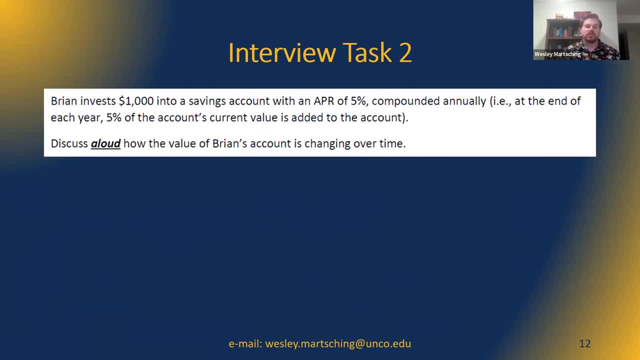 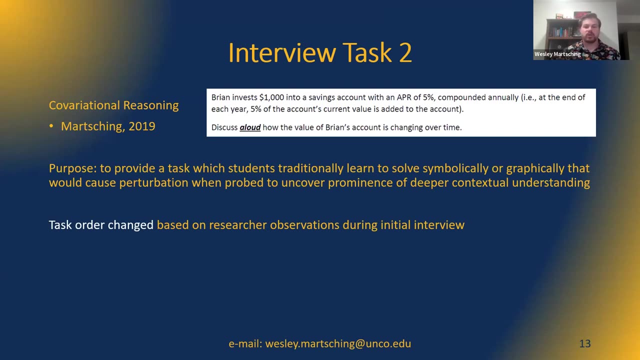 research, And this is one of those tasks where I noticed that students will create different representations for it, but the way they talk about the context through these different representations will vary, And so, with these two participants, I did change the question order for the second task. One question had the participants discussing aloud how the account 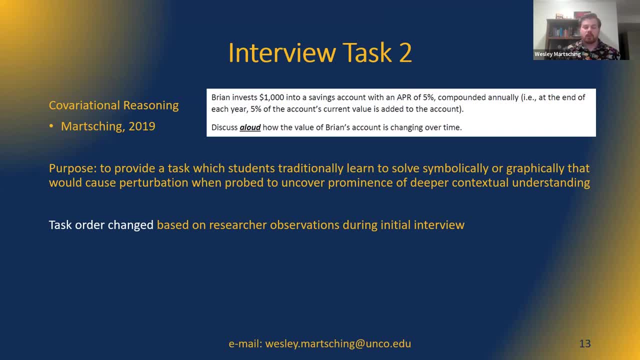 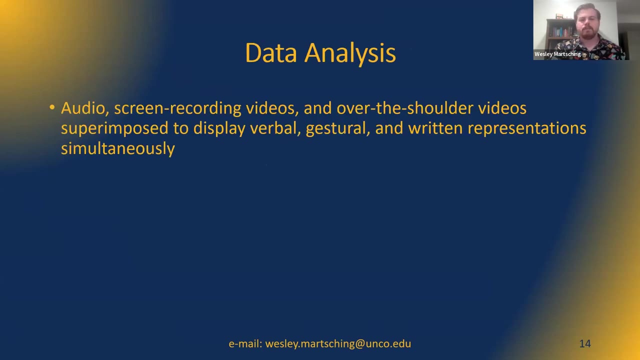 value is changing over time. The other one had them graph it or model it through graphing And I did change this task order because I wanted to see how their reasoning changed when the order changed. For my data analysis I took the audio, the screen recording videos and over-the-shoulder. 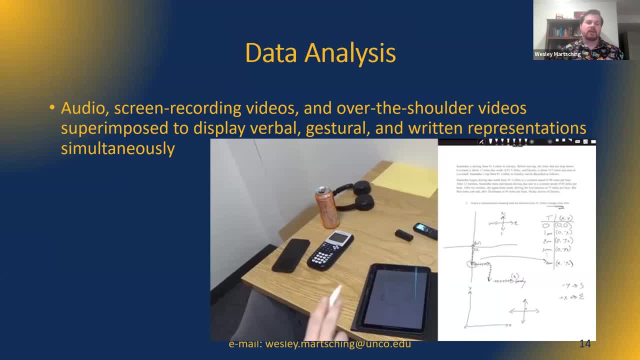 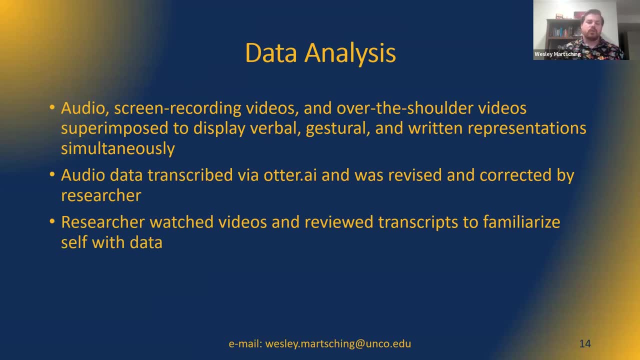 videos and I superimposed them so that I could look at the verbal, gestural and written representations at the same time. I used Otterai to transcribe the audio And I used disguiseai to transcribe the audio. I used disguiseai to transcribe the vision. 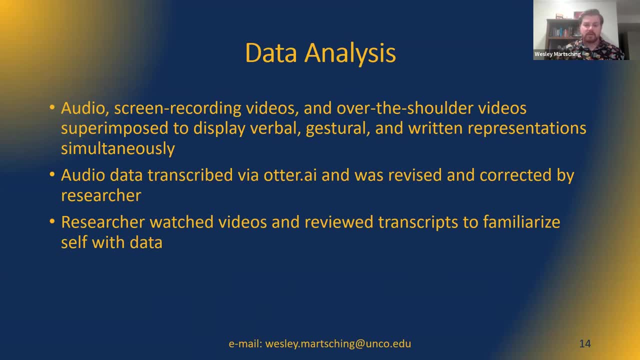 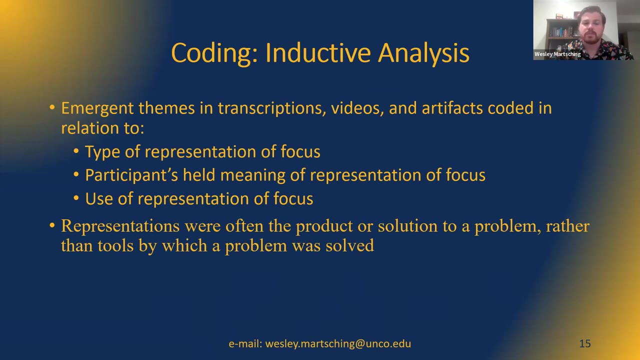 And then I went back through and corrected them myself to make sure that everything was okay. And then I rewatched all the videos and reviewed the transcripts to familiarize myself with the data before coding. I used inductive analysis to look for an emergent themes in the transcriptions, videos and artifacts And, in particular, I focused first on what type of- or yeah, the- representation. that was a focus in a moment. 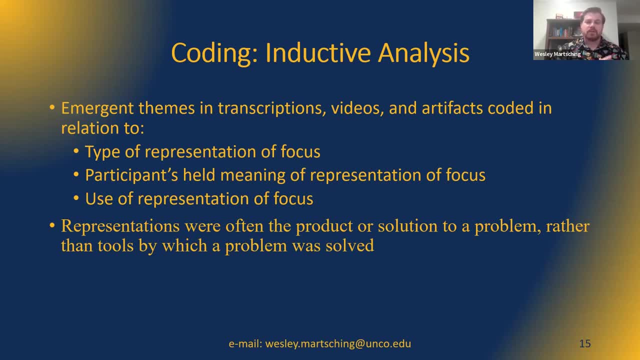 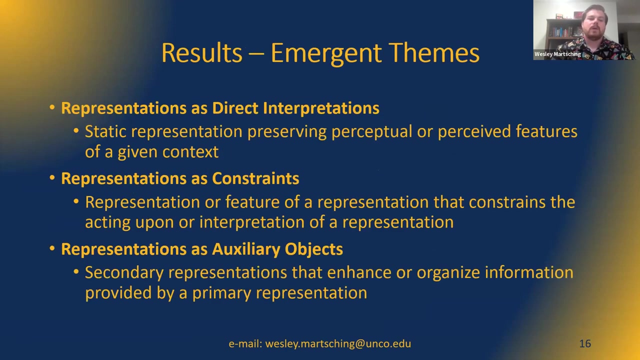 What the meanings the participant had of this representation was and how the representation was being used in that moment. And I do want to highlight that this is different from the work that Stylianou did, because here the representations are often the product or solution to a problem and are not just tools being used to mediate the problem solving process. 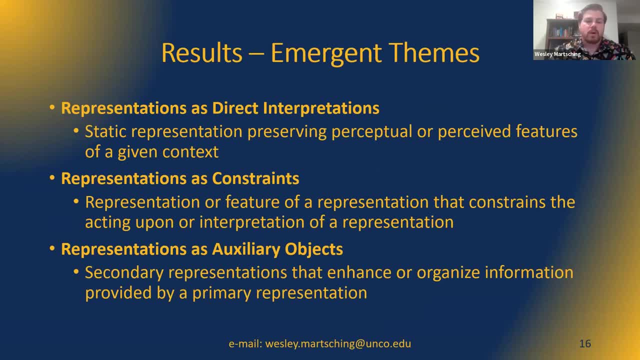 The three themes that came out of my data analysis were representations as direct interpretation, Which is where the students would create a representation to exactly model what it is that they were perceiving Representation as constraints, which could be used to constrain the students reasoning or constrain the interpretation of another representation that they'd already created. 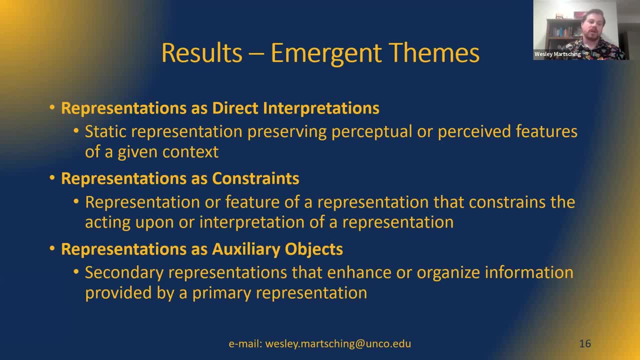 And representation as auxiliary objects. So sometimes the initial representation that a participant created did not convey all the information they wanted it to. So the initial representation that a participant created did not convey all the information they wanted it to, So they might create a secondary or tertiary representation that could add additional information to their original representation. 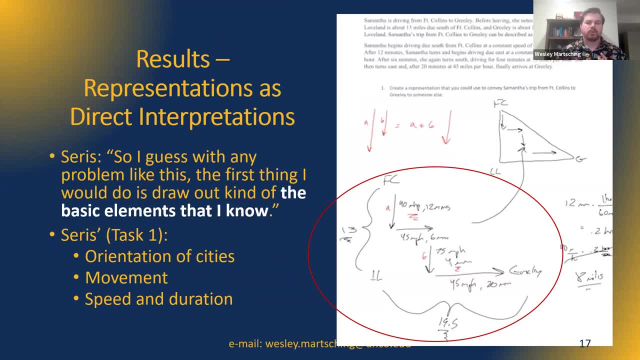 So I'll go through some examples of each of these themes. The first one has Ceres responding to the first task, which said: create a representation that you could use to convey the car's trip from Fort Collins to Greeley to someone else. And Ceres said: you know, I basically just drew out the basic elements that I know. 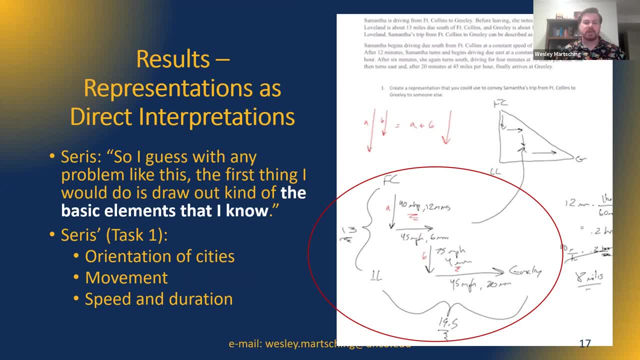 And Ceres said: you know, I basically just drew out the basic elements that I know. He drew these vectors that depicted the car's trip from Fort Collins around Loveland to Greeley. Next to each of these vectors he wrote out how fast the car was traveling, how long it was traveling for, and then out to the left and below he illustrated the distance between each of the cities. 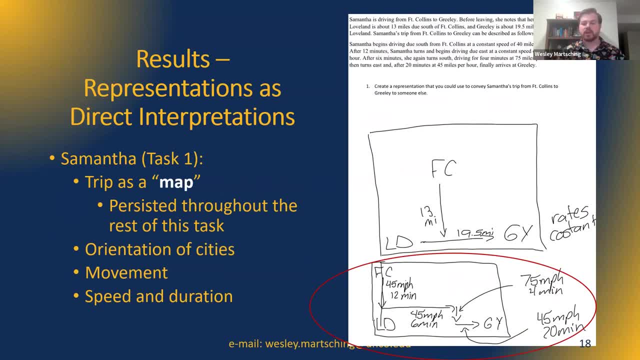 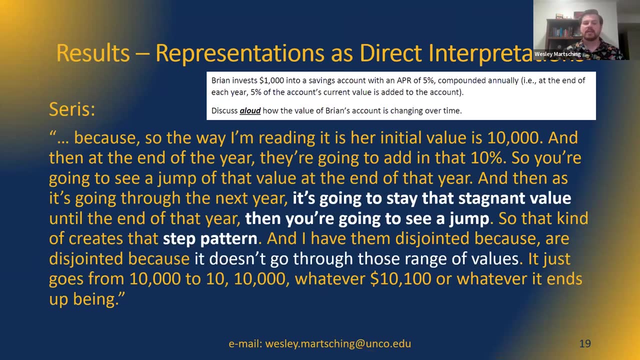 Similarly, Samantha created this map that also depicted the orientation of the towns And showed the speed and duration of each leg of the journey as well. For the compound interest task, Ceres was asked to reason verbally about the task before creating the graph. 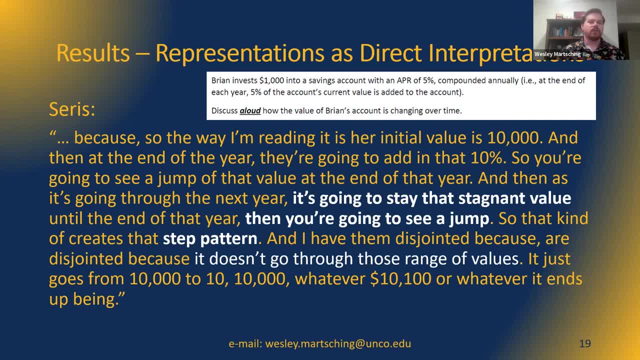 And Ceres immediately jumped to this kind of step value depiction. He said: you know, the amount is going to stay at that stagnant value. You're going to see it jump And you're going to kind of see this step pattern. It doesn't go through these range of values in between. 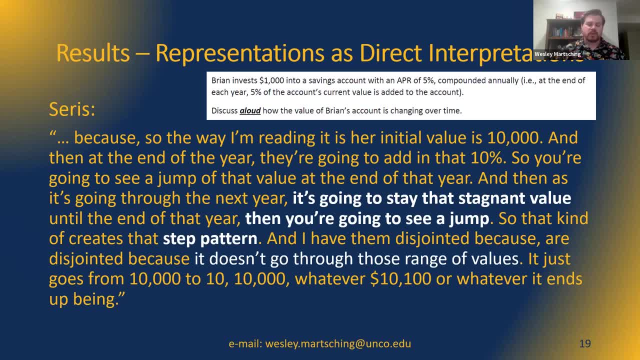 It just kind of jumps up. And so for Ceres, reasoning about this task aloud and then creating it on the graph meant that he wasn't relying on any algebraic formulas or anything else to create his graph, He just drew it strictly from his interpretation after reasoning about it verbally. 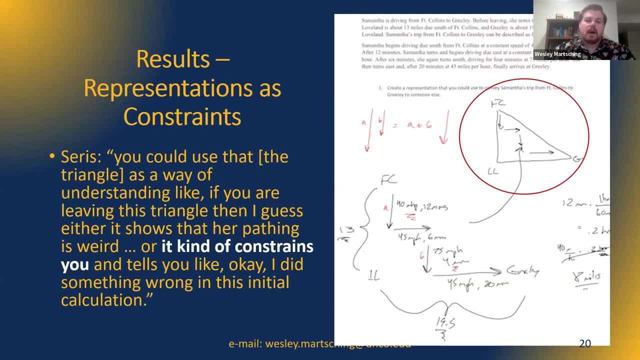 Looking at representations as constraints Again. going back to Ceres first, he kind of took that original depiction of the car's travel and situated it within this triangle. So because Loveland is basically due south of Fort Collins and Greeley is due east of Loveland, he said that if at any point in time the car travels outside of this triangle, it means that either he did something wrong or it meant something was wrong about the context. to begin with, 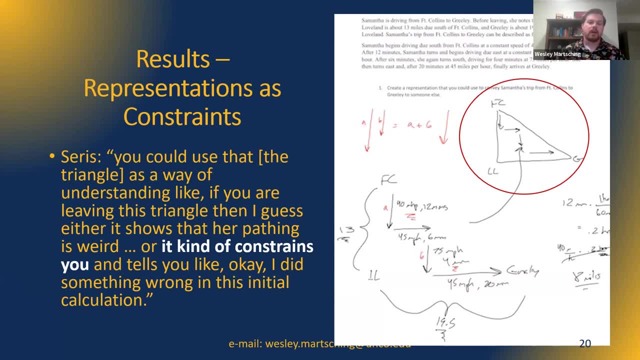 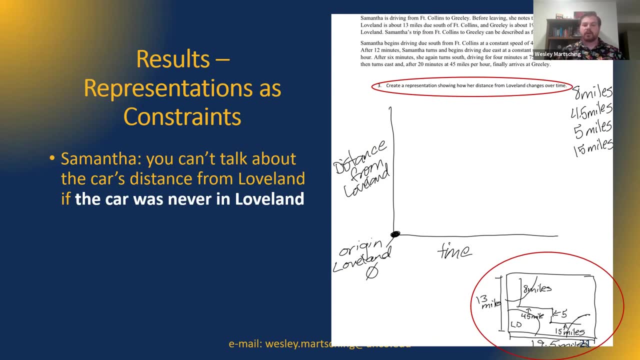 So it kind of constrained his reasoning and was used as a way to check what he was doing. Samantha also continually referred to her map and also used this reasoning about the orientation of the cities to talk about what she was doing. And in this example- this third question for task one- the participants were asked to create a representation showing how the car's distance from Loveland changed over time. 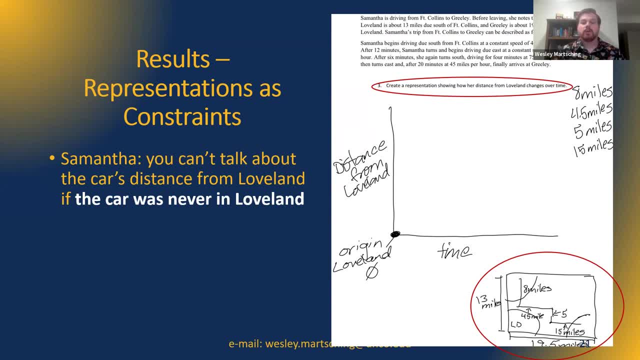 For Samantha, this- her interpretation of this task- also produced a representation of the car's travel, So she was able to tell if the car was moving in the right direction or in the left direction. And so she was able to tell if the car was moving in the right direction. 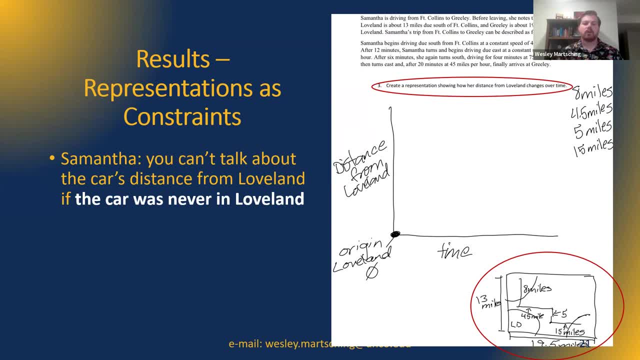 And she provided a constraint For Samantha: she couldn't talk about how the car's distance from Loveland changed over time, because the car was never in Loveland. So we see this additional constraint where Samantha said: well, this question is nonsense, because her original representation clearly showed that the car was never in Loveland. 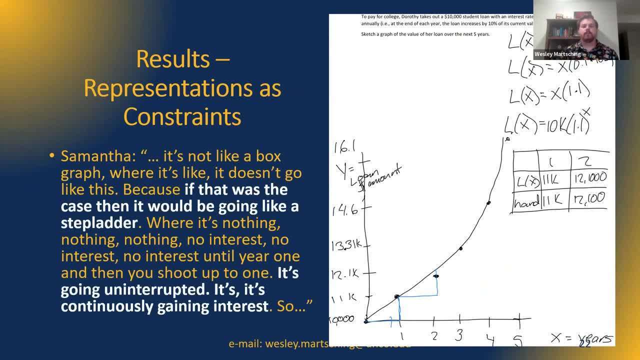 We can't talk about that relationship. And on the compound interest task, Samantha engaged in the task first before being asked to reason verbally. asked to reason verbally about it. So she created this algebraic representation that you see in the top right, checked it using a couple values in a table, said okay, this is the function. Now I'm 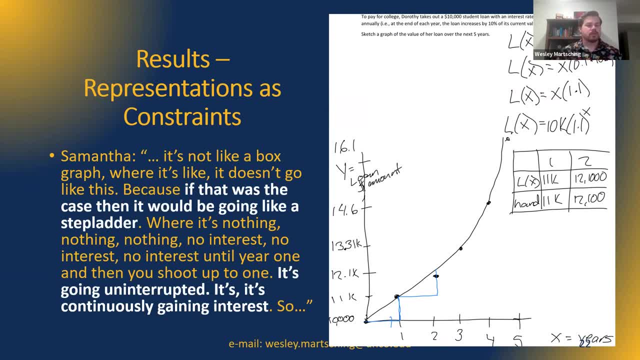 going to graph it And she created this smooth trace. When she was asked to reason about it verbally, she, similarly to series, started talking about this step-like pattern, which you can see that she started to draw in blue, But she said: well, that doesn't really line up with the. 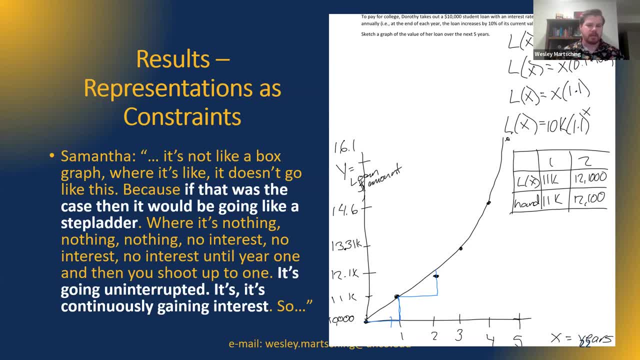 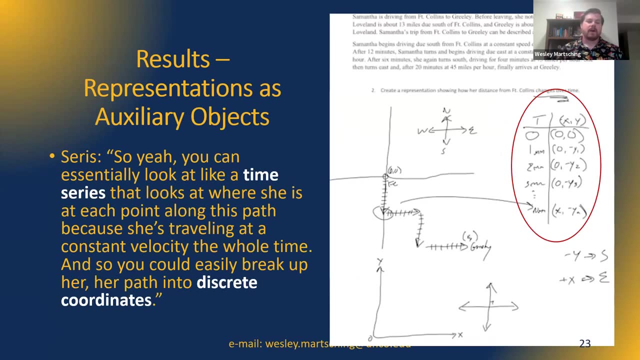 representation that I already drew, So it can't be this step-like pattern. She actually concluded that the original context must be wrong, because the amount in the account has to be growing continuously to match her graph. And finally, looking at representations as auxiliary objects, 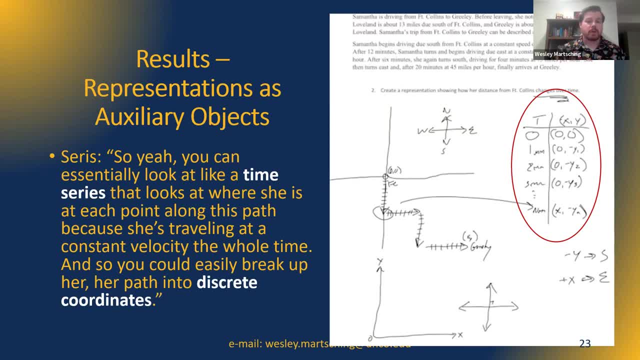 for this question. the participants were asked to create a representation Showing how the car's distance from Fort Collins changes over time series. said well, I drew the trip in two dimensions. I can put that on an X- Y axis and I can show what's happening. 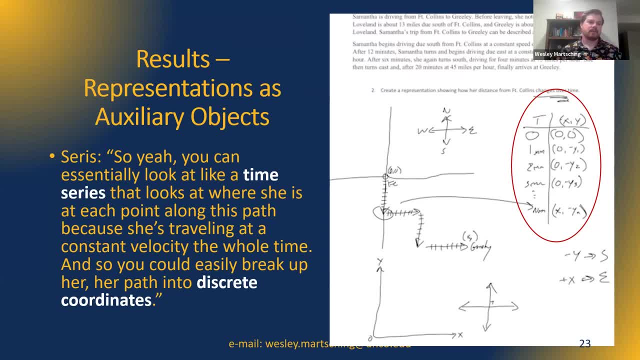 that way. But he said this doesn't really have any value of time that we can see. So I'll create this other representation, this time series, where I can talk about these discrete sets of points along the trip And I can talk about what the vertical and horizontal distance traveled actually. 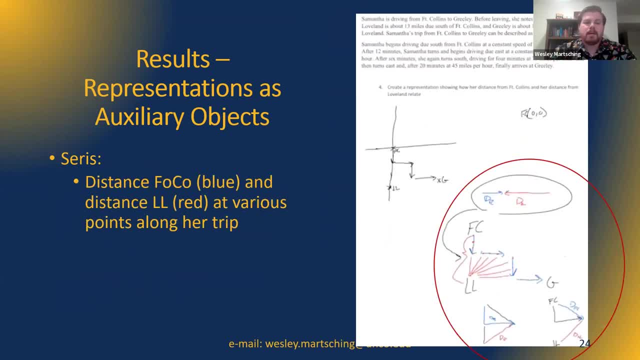 is On a later question which had the participants represent how the distance from Fort Collins and the distance from Loveland relate. series color-coded two distinct vectors. The blue vector that you see actually represents how far the car is away from Fort Collins at any discrete point. 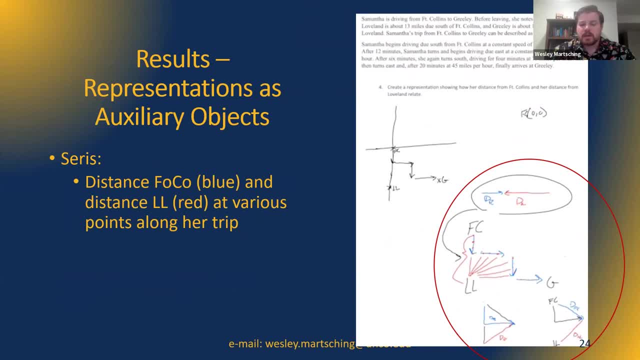 And the red vector represents, or the red segment represents, how far the car is away from Loveland at the same points in time. So again that coordination of the two values simultaneously, And in this case he used these additional red and blue vectors to show how that distance was. 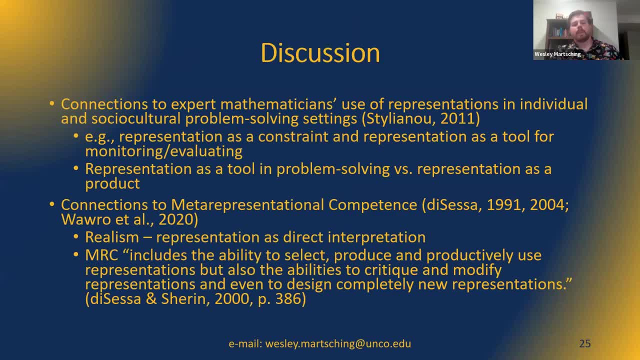 changing from both cities. I do see connections between these three, these three things, Names and other things, in the literature, especially Stelliani's research. So the representation as a constraint really kind of resonates with that representation as a tool for monitoring and evaluating. But again I do want to highlight that in that research 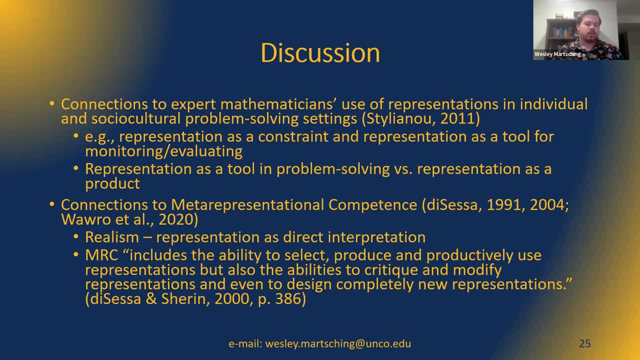 the representations were a tool in problem solving, And here the representations are the products or the solutions themselves. There are also, again, those connections to meta-representational competence. So looking at how students can judge their own representations, how they can critique them and how they can create them. 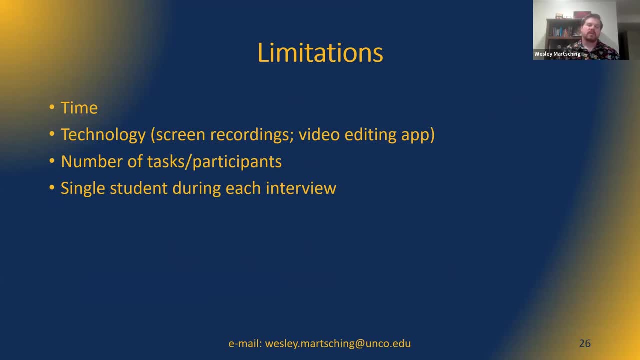 There were quite a few limitations. Obviously, I would have loved to have had more time with each participant, maybe two interviews. Technology was sometimes an issue, especially with the screen recordings. It seemed like my iPad was recording in discrete intervals as well. 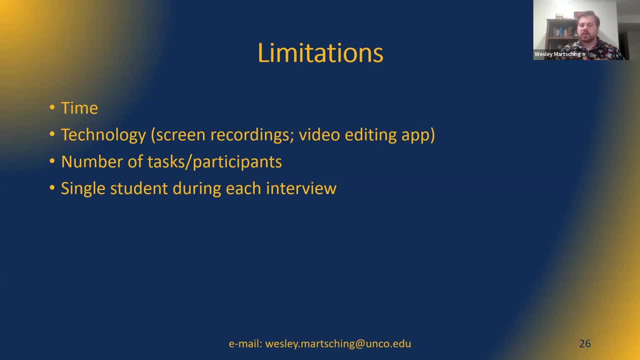 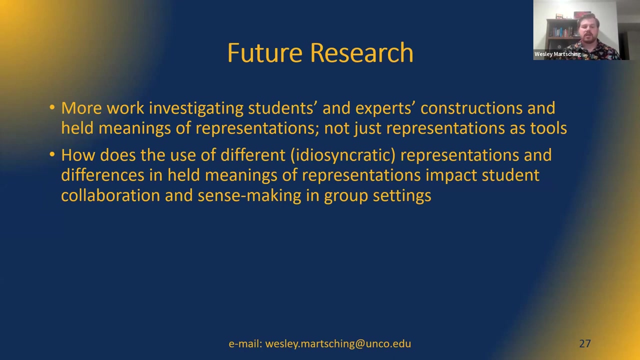 There were only two tasks and two participants. I would love for those numbers to be higher as well- And I only interviewed one participant at a time. So I do believe that future research should continue to look at representations in this way And, in particular, I think it should look at how different idiosyncratic representations and how these differences in held meanings impact student collaboration. 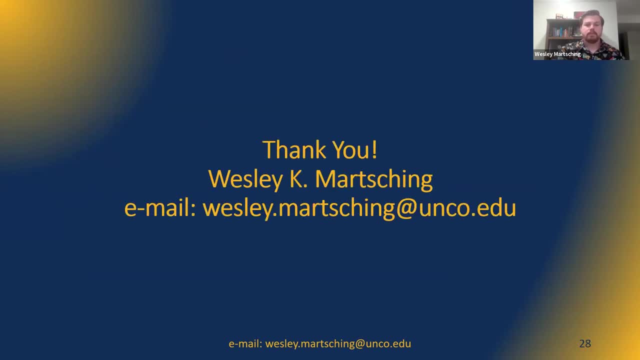 And, in particular, I think it should look at how different idiosyncratic representations and how these differences in held meanings impact student collaboration. So thank you all for attending. There's my contact information if you would like to reach out. Thank you, Wesley. Does anyone have any questions for him? 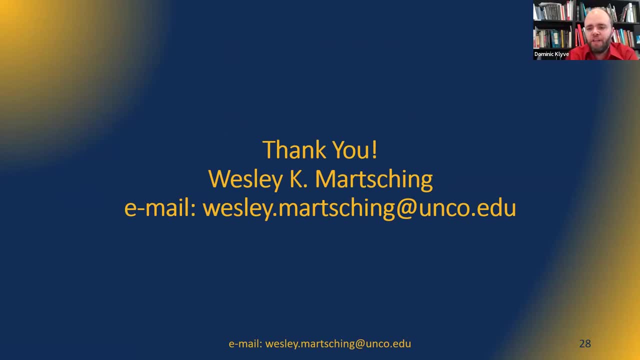 I have a question. This is sort of asked from a position of ignorance as someone who doesn't do education, research. What's the benefit of the overhead camera? So I feel like when you showed us a picture of their work, I got a really good picture. 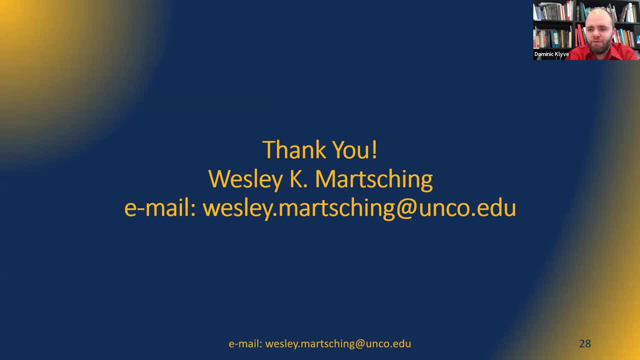 I think it's a really good understanding of what they did. what more do you get from it, seeing it sort of play out in time? So being able to see the screen recording play out in time shows us you know what they are creating at any point in time. what representation you're talking about. 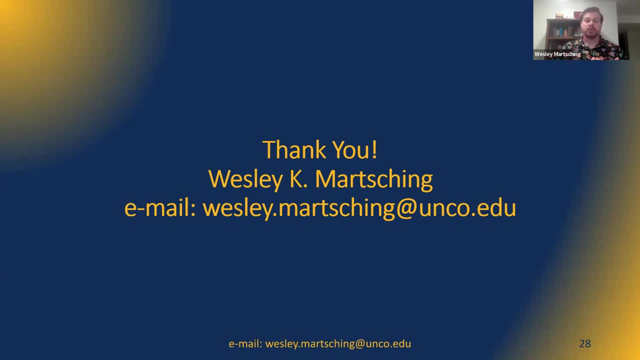 The over the shoulder camera also shows us what kind of gestures they're making. So that didn't come up a lot in this research, but if they had have been making these very like particular gestures, that could also be considered an external representation. So that's just something I tend to do in my research is using that over the shoulder camera. 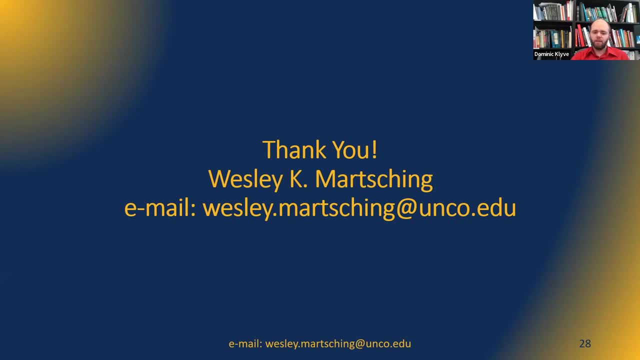 That's cool. Also, that was interesting stuff. I hope you keep doing more of it. Thank you, I think it's going somewhere. Yeah, I love it. It's great, It's interesting. I love seeing it and working with the students. 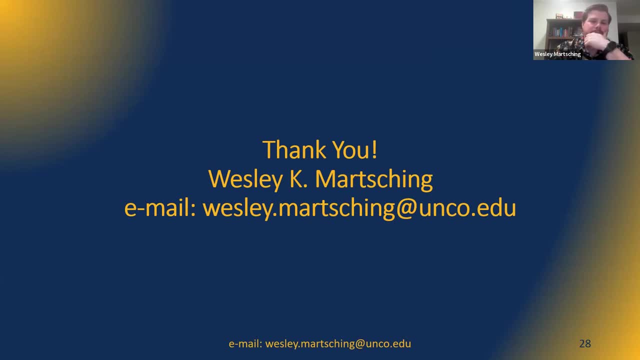 Other questions? Um, hey, um, obviously that was a really interesting. um, I was wondering, like, what overall students interactions and representations look like over the semester and how that relates to how they use them in this kind of tasks. 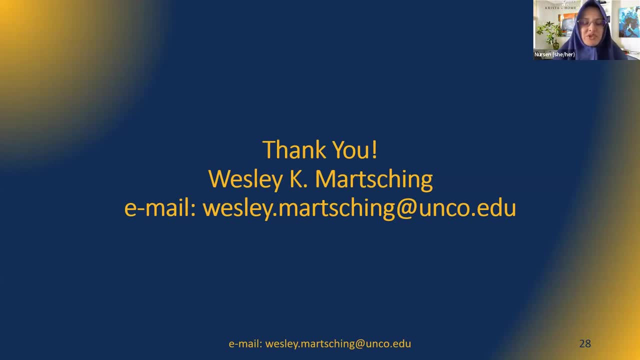 I just always just curious. I know that's not part of your research, but I was just wondering overall how their experiences impact their reasoning and engagement with for presentations. So I think that would also be a great follow up question for this study. I was not the instructor of record for that calc one course, So I actually don't know what kind of content they covered, especially right before. 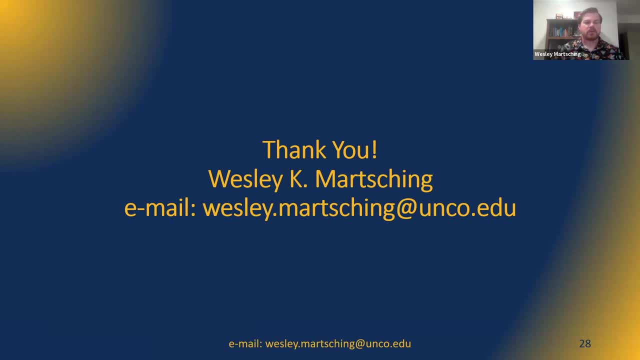 these interviews. That is something that I myself wondered about, especially in seeing in. seeing like series is time series, but I don't have access to that information. Thank you, Okay, looks like we're about out of time. If you have more questions, you can email Wesley for them, But thank you for all that great information that you share with us. I've posted in the chat What the